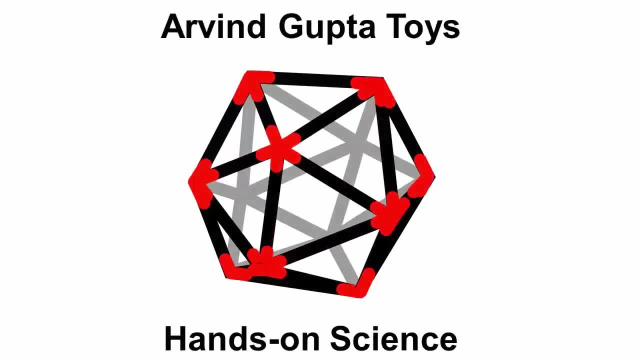 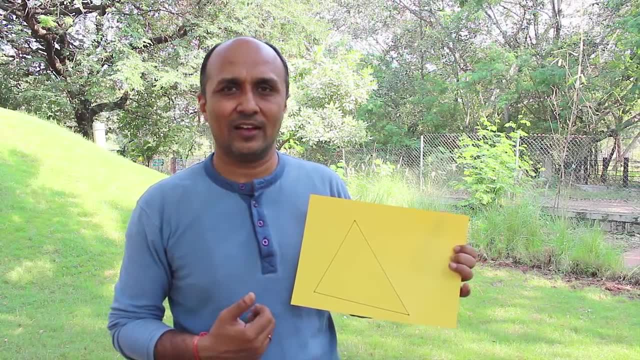 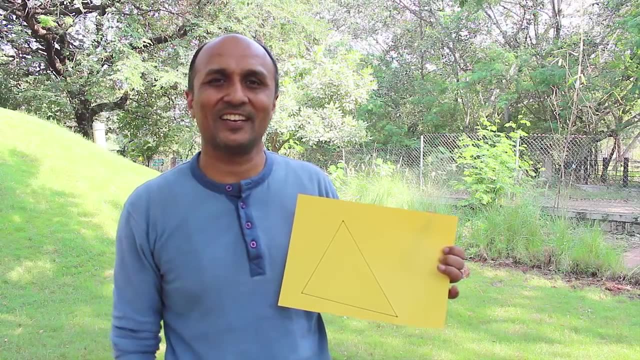 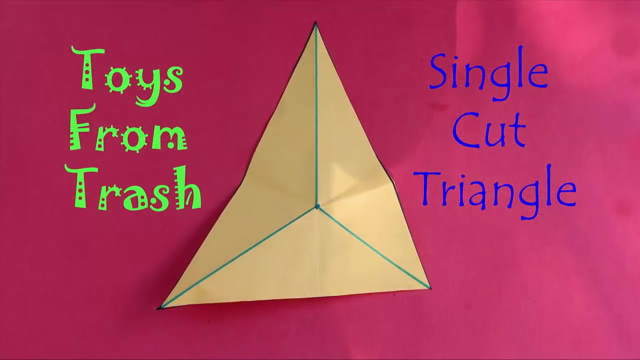 This is any triangle and in fact it's a scalene triangle, which no three angles are equal. but can you cut this triangle out of this paper with just one single cut in a straight line? It's a wonderful activity and we are going to see how Single cut triangle and all we need for this is. 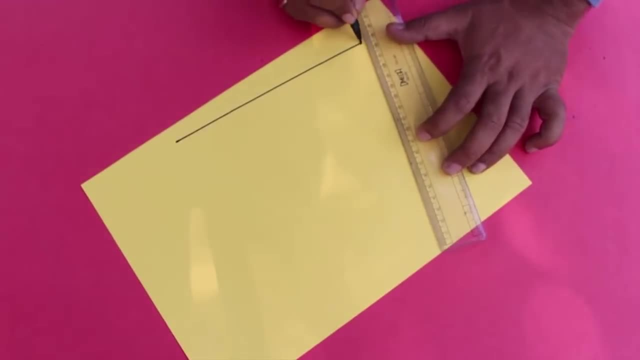 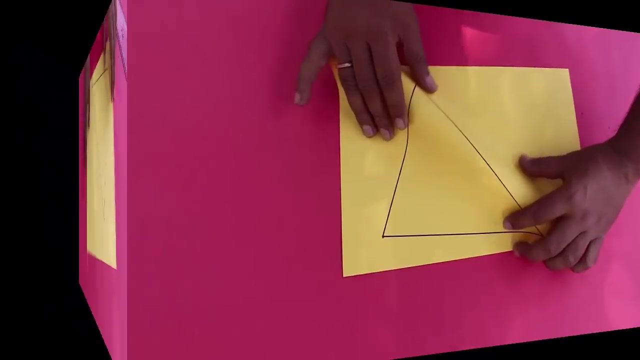 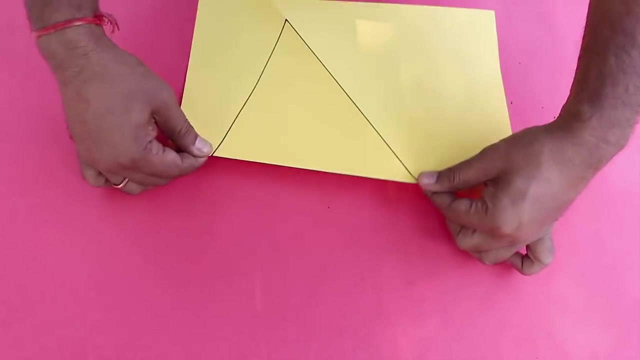 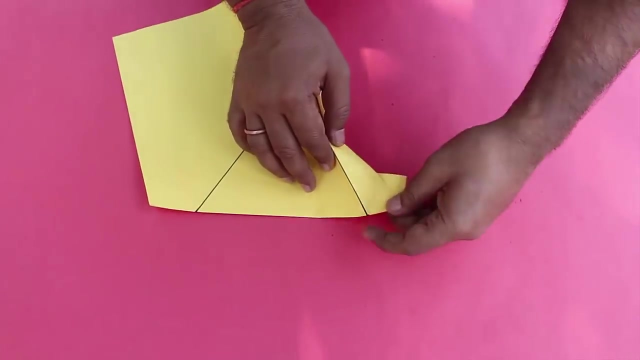 is just a simple piece of paper, pen and a scale. First we will draw any scalene triangle where all three sides are of different length and hence all three angles are also different. We will first fold the paper along the sides of the triangle and then, once we are done with that, we will place one side on top of the other. 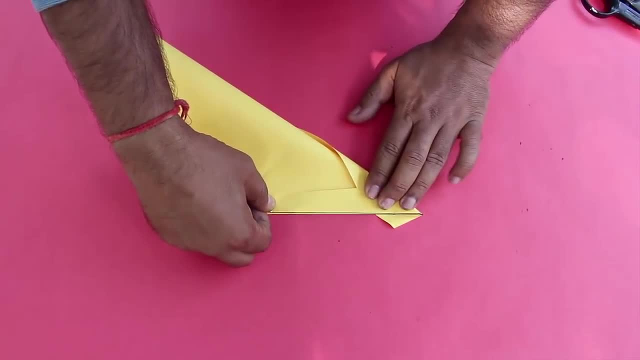 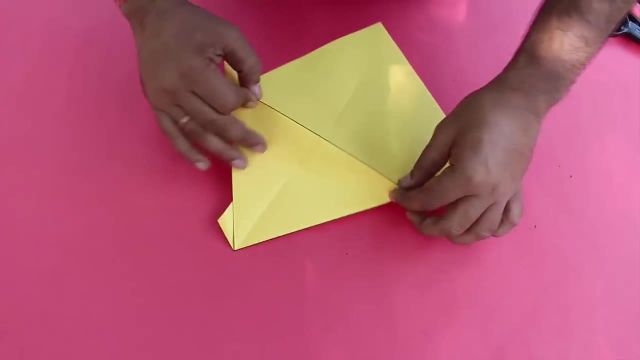 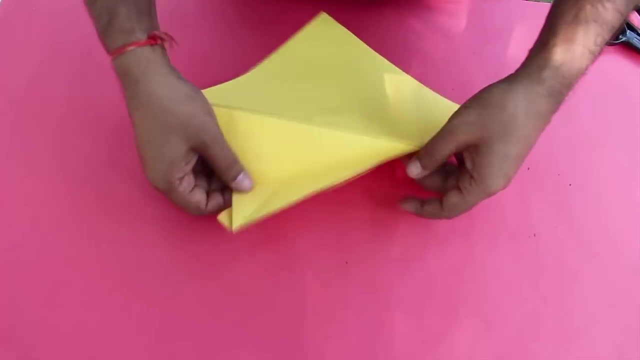 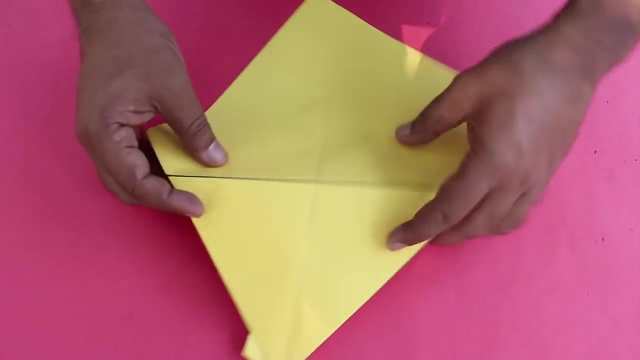 thereby dividing the angle in two equal parts. The line of the fold is called the angle bisector. This line divides the angle in two equal parts. We will do the same for the second angle, and this line again divides the angle in two equal parts. and these two lines meet at a point which is called the in-center. 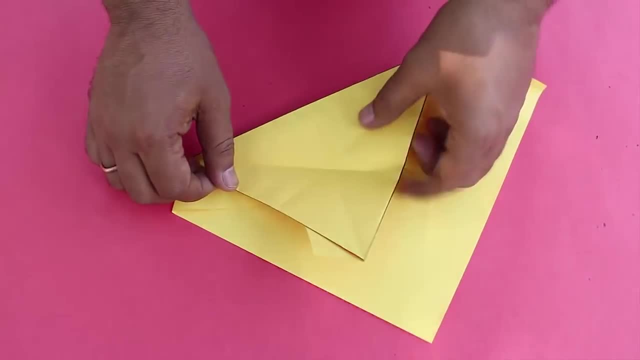 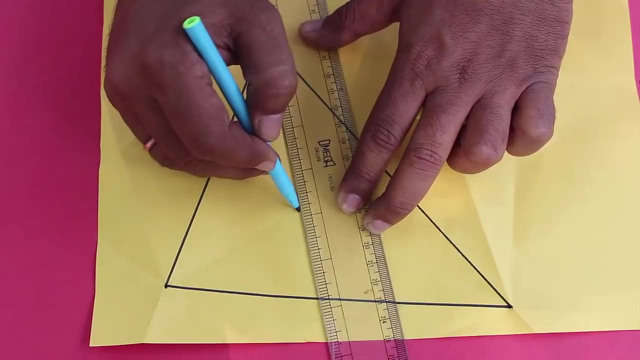 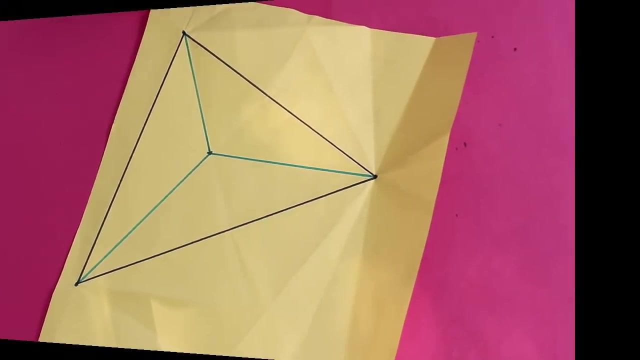 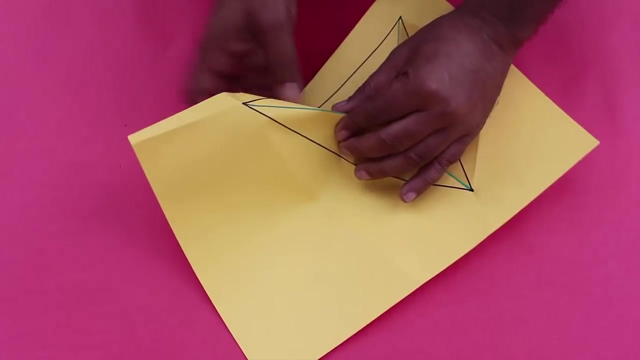 and when we divide the third angle, we find that the third angle bisector passes through the same point, which is called the in-center of the triangle. Now we will draw all these bisectors, the angle bisectors of the triangle, and fold the triangle along these angle bisectors. It is like dividing the triangle in three. 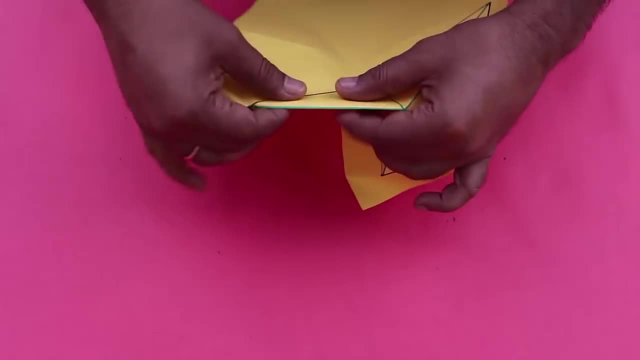 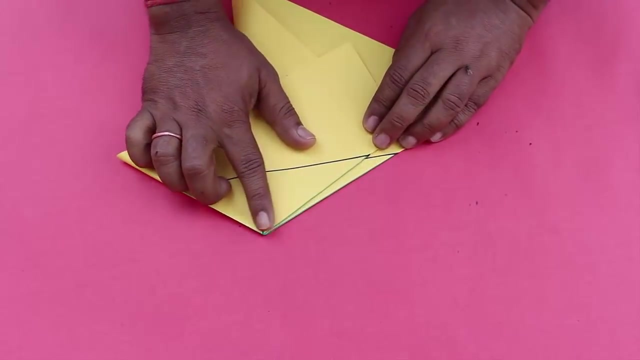 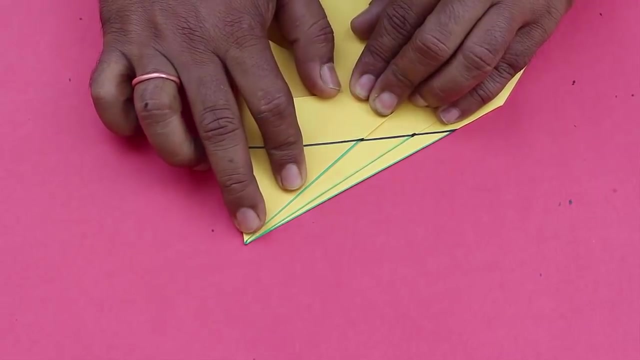 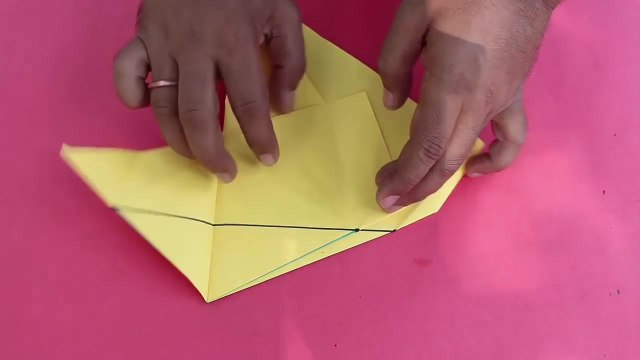 parts or three petals which overlap each other, And when we fold such that the bases meet, it is almost like drawing a perpendicular from the in-center to each side of a triangle, and since it's an in-circle, which means that the radius of the circle from the in-center to each of the side is the same, that's why all these three petals.